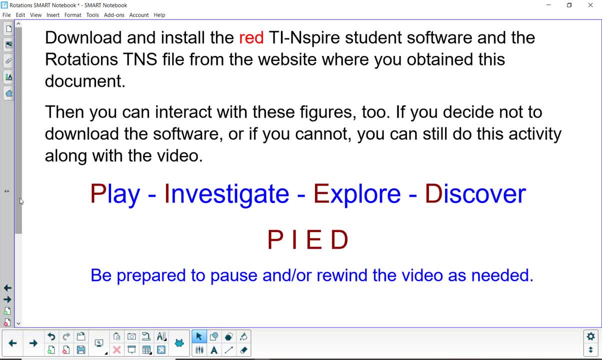 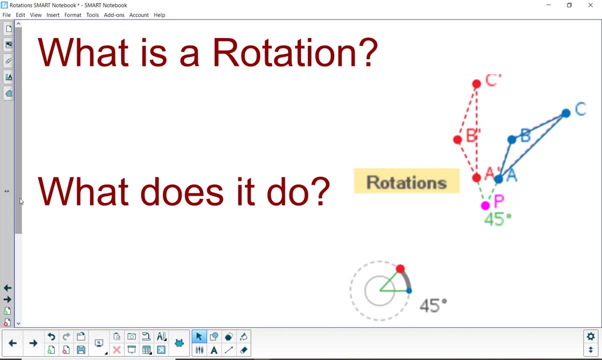 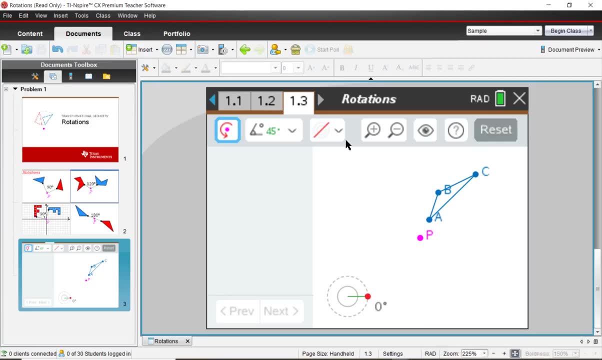 Be prepared to pause and to rewind the video as you need to do so. So let's first look at what is a rotation. What is a rotation and what does it do? So we'll go to the TI-Nspire technology. Here we have the TI-Nspire software open and the file rotations and we've moved to page 1.3.. 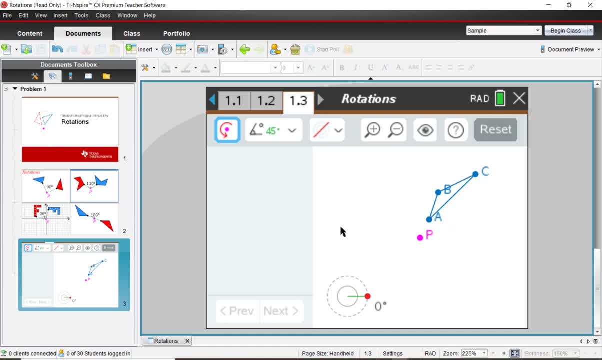 So we're going to rotate triangle ABC about point P through an angle of 45 degrees. So to do that, here is the rotate icon. So let me go ahead and click on that and observe what happened on the screen. So pause this if you need to. what's going on on the screen? 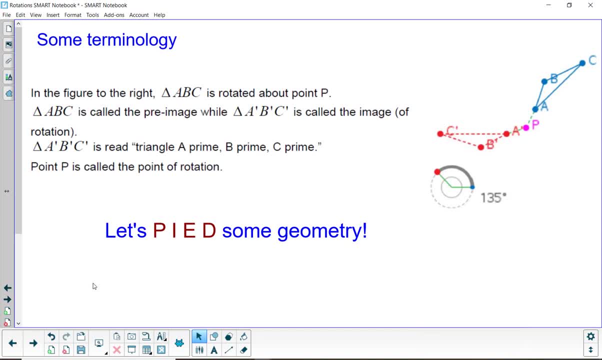 A quick review of some terminology. In the figure to the right triangle ABC, the blue triangle is rotated about point P, pink point P. Triangle ABC is called the preimage, while the red triangle- red triangle A', B', C' is called the image of rotation. 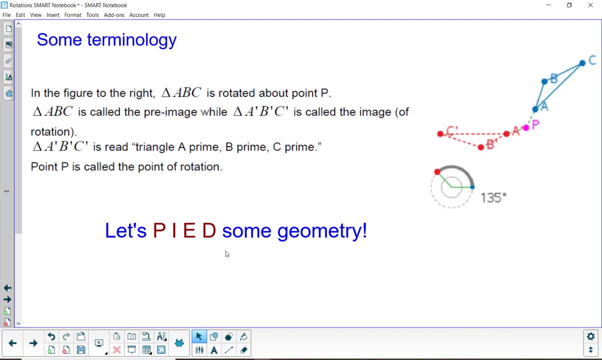 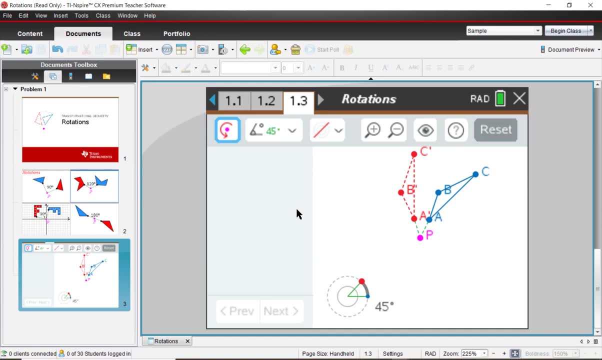 So let's play, investigate, explore some geometry. Going back to TI-Nspire, notice what has happened here. We have moved triangle ABC rotated about 45 degrees. So let's click on the rotate icon and rotate another 45 degrees. 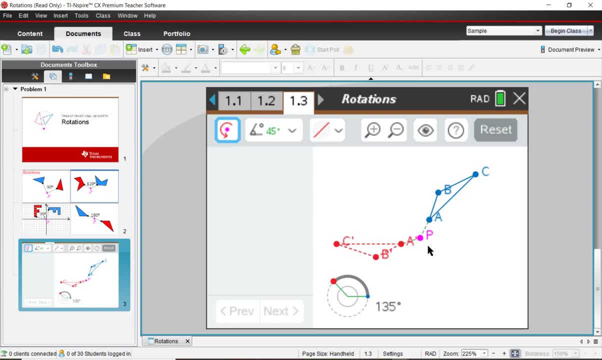 And another 45 degrees, For a total of 135 degrees. Let's do this again, only this time I'm going to go over to tools, click on templates and do the first template tour. So tools templates tour. 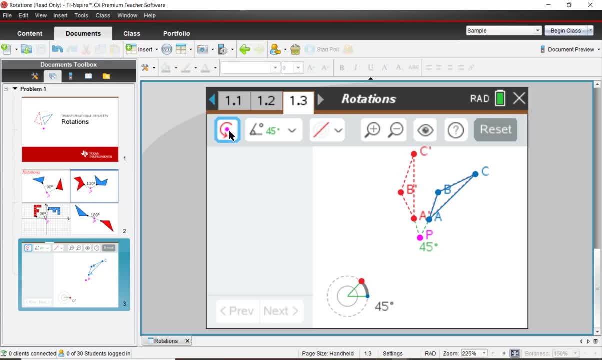 And again I'm going to rotate triangle ABC about point P, 45 degrees, And then again and then again, And you'll notice what's happening is the previous image is shown as kind of ghosted kind of out, And so that we can pay attention to that. 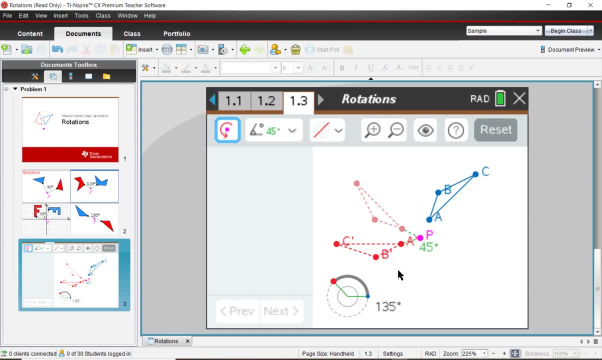 But the original triangle has been rotated 135 degrees about point P. So here's what I'd like you to do. I'd like you to decide: what do you notice about the original preimage triangle and the image triangle? There are several things that hopefully you're noticing about those two triangles. 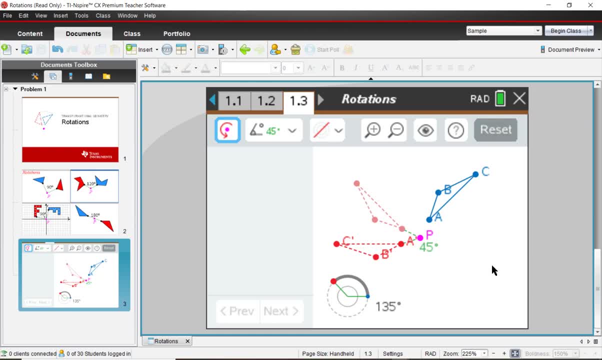 So please pause the video and think about that. It appears that these two triangles are congruent, But that's only for one pair of triangles. We really should try to investigate more. So with the software, I'm going to go ahead and click on grab on point A and pull it. 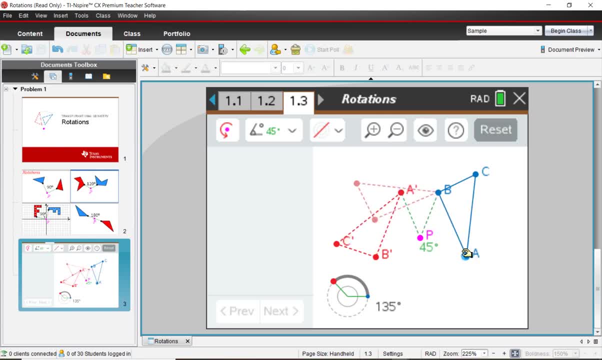 And as I do that, you can see several things change. Do those triangles still seem to appear congruent? I can grab point B and play with that And point C. I can even grab the entire triangle And see what happens, And we can even grab point P and move that. 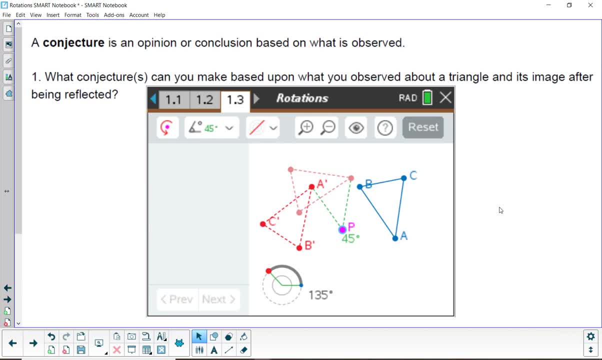 So let's turn to number one, on the PDF Reminder that a conjecture is an opinion or conclusion based upon what you've observed. So, based on what you've observed in number one, what conclusions can you make about a triangle and its image after being reflected? 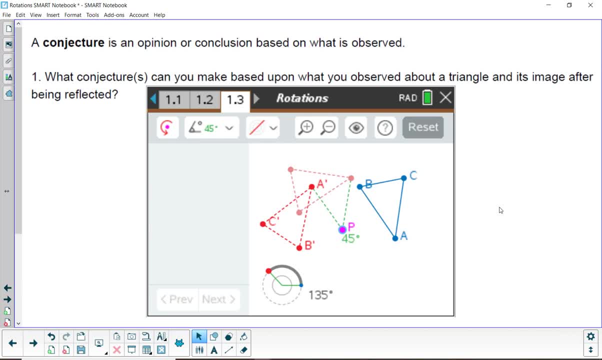 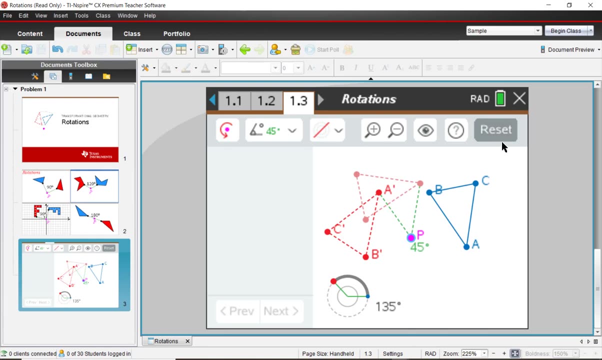 So you can do that on your PDF. You can write the answer down on your paper. You can copy it on your paper Whatever works best for you. Please pause the video to do this now. Let's try other angles of rotation before we finish our conjectures. 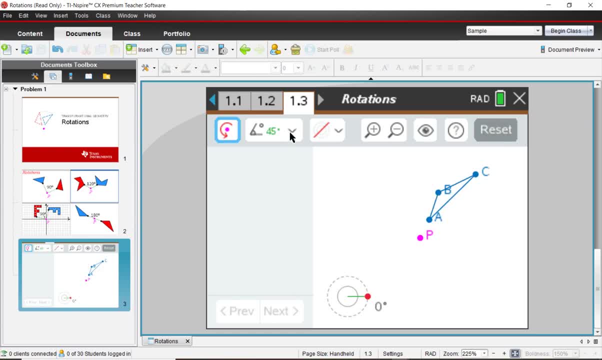 I'm going to go ahead and click on reset And here's the angle drop down measure. So let's go ahead and click on, let's say, 30 degrees, And let's go ahead and rotate that triangle about point P: 30 degrees. 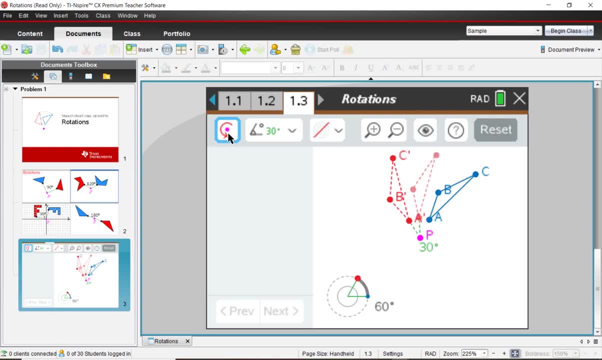 Those triangles seem to be what your conjecture said: 30,, 60,, 90, and so on. Again, grab, move things. It still seems to be true. The angles are different. Continue to rotate. Continue to rotate. 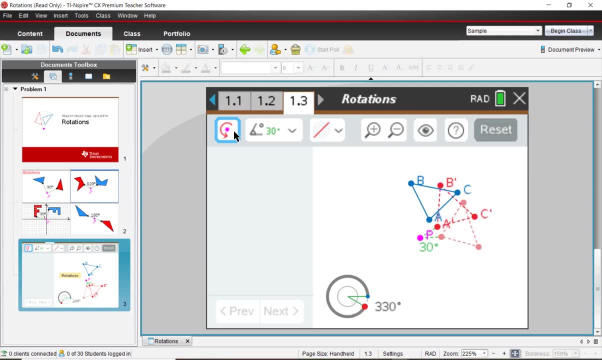 And I'll continue to rotate until I get to a rotation of 360.. And what do you notice about a rotation of 360? A rotation of 360 degrees lands back on the original pre-image triangle And so far I think our conjectures seem to be true for multiples of 30..